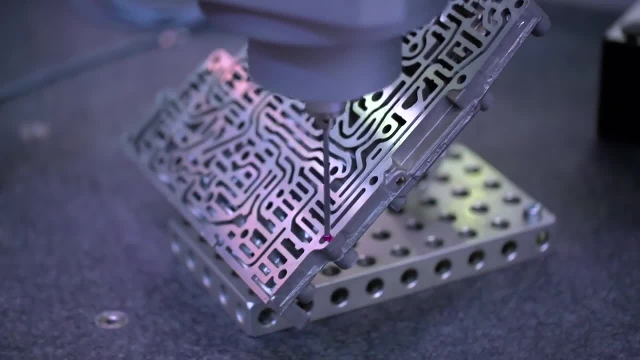 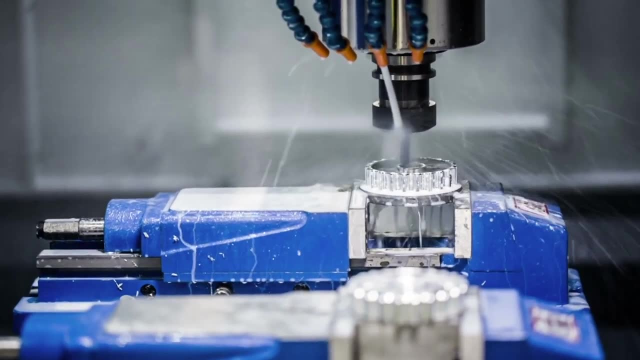 process is used to create your design. Certain machines will have a maximum tolerance and if you need a tighter tolerance then you'll need to find a new machine to create your part. Tolerances naturally come out of clearances, For example. you might know you must maintain. 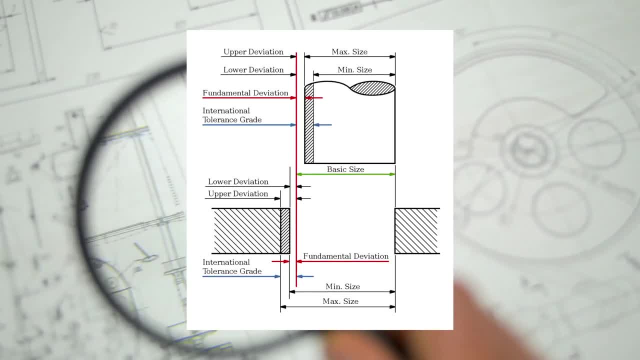 a clearance of a part of a machine. if you have a tolerance of a part of a machine, For example, you might know you must maintain a clearance of a part of a machine if you have a tolerance of 2 centimeters plus or minus 0.1 centimeters. This clearance would likely be there to avoid. 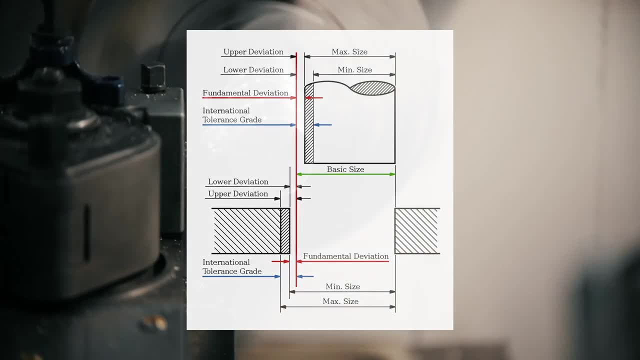 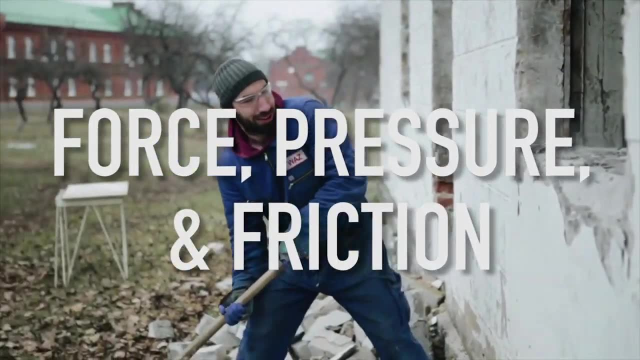 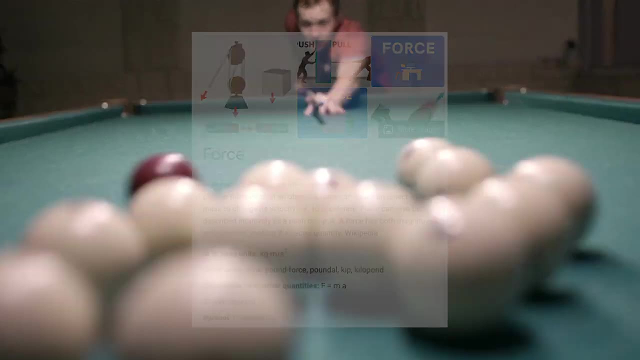 friction or to avoid the part catching another moving part. The tolerance of this clearance value would be the 0.1 centimeters. Next, let's move on to force, pressure and friction. Forces are the measure of mass times acceleration. They're what determine our everyday life. 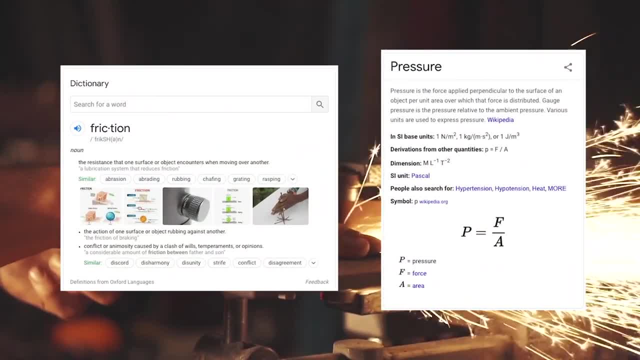 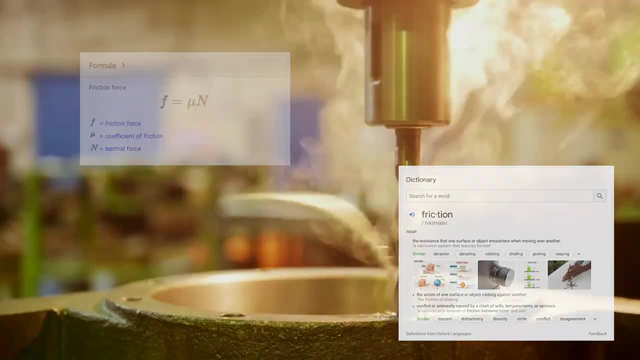 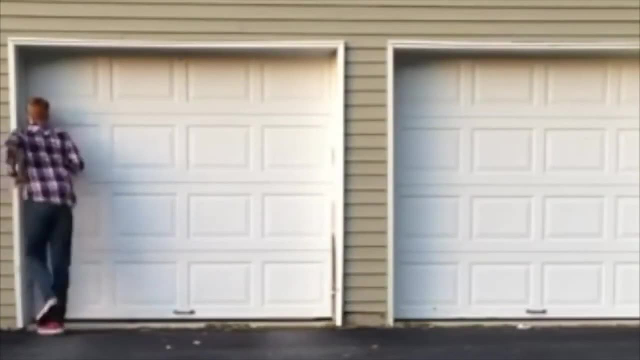 Friction and pressure are both types of forces, often the most discussed, Focusing in on the latter. friction is the reason everything works the way it does. If you actually want to find out what happens if friction were to disappear, we have a video about that linked in the upper right here. but back to this video. 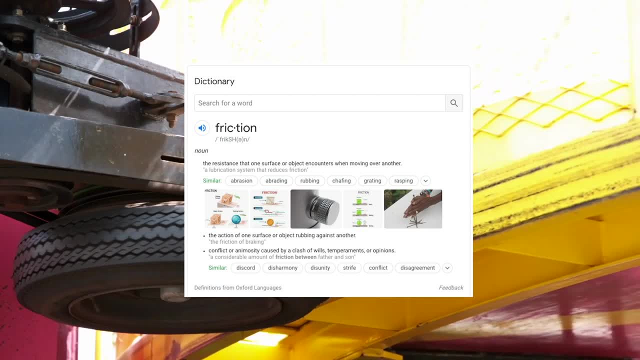 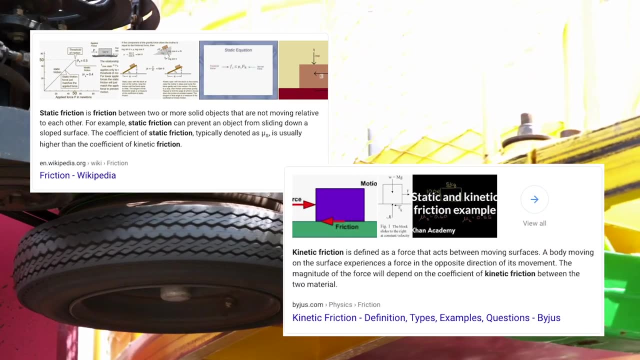 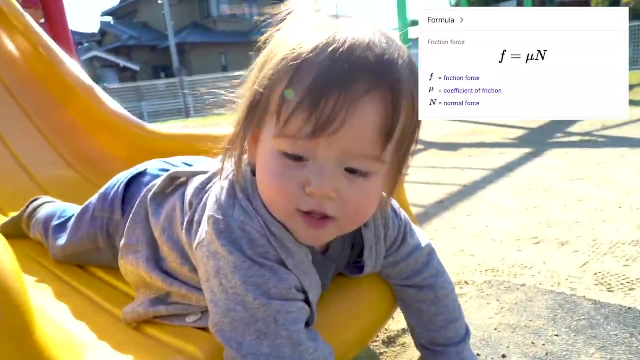 Friction is a restricting force exerted on an object when, in contact with another object, There is kinetic and static friction, which usually have different coefficients or values for a given surface. Essentially, friction is a resisting force that can be variable based on surface properties, velocities and accelerations. Pressure is similar. 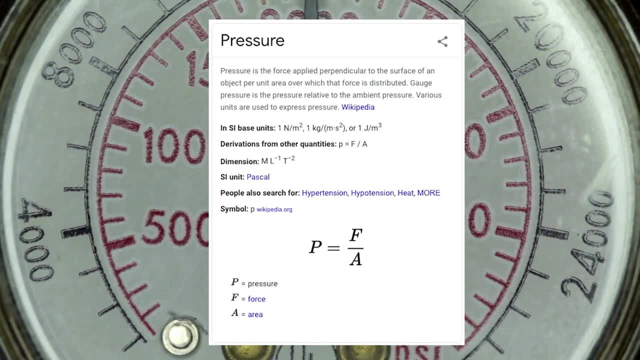 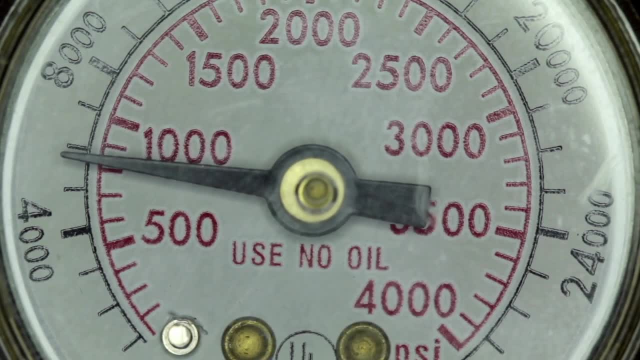 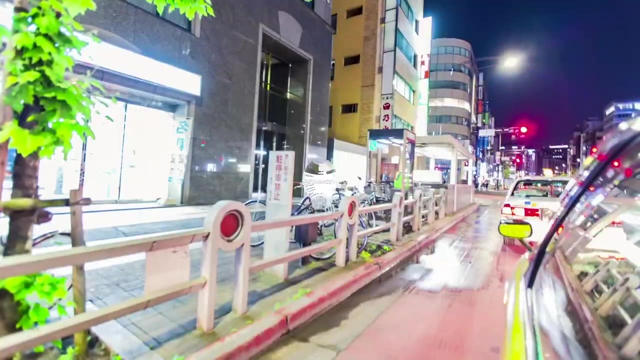 to friction in that it's a continuous force exerted against an object when something is in contact with it. It's also presented as a force on a specified area. Think in pounds per square inch, psi. Next, let's talk about velocity and acceleration. Velocity is the speed of something in a given 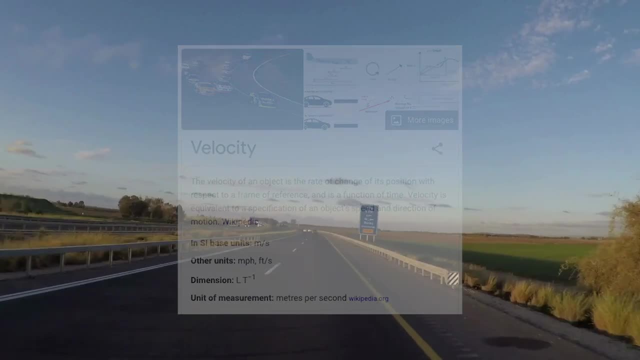 direction. This means that velocity is a vector, meaning that it's both a numerical space or velocity of the object. This means the velocity of the object is the same as the velocity of the object itself. So, for example, we get a speed of 1, which means that velocity 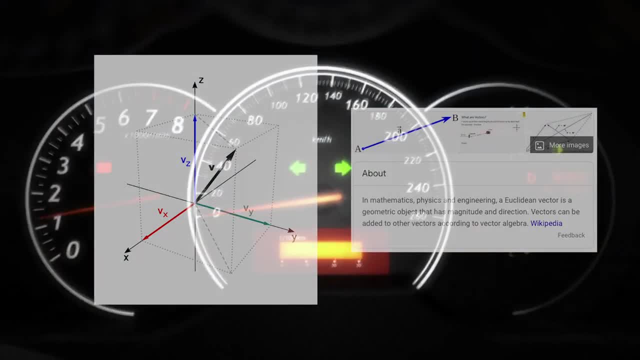 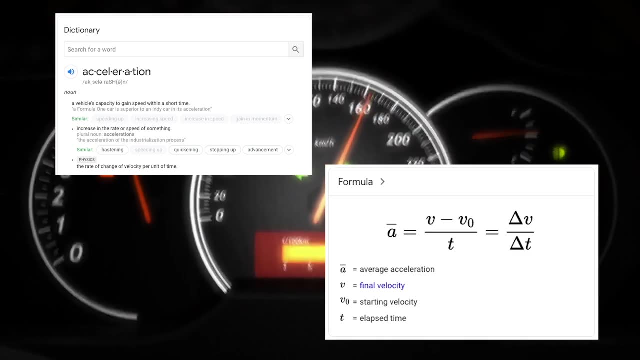 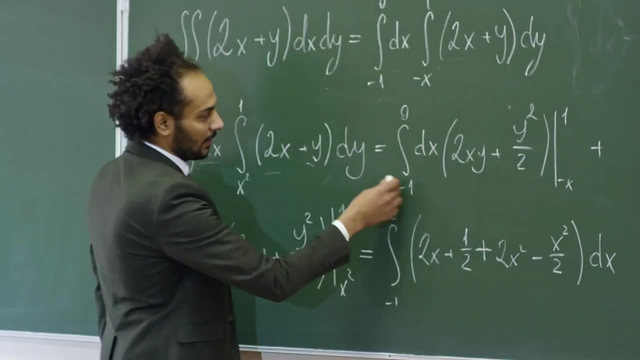 speed value and a directional value. Acceleration, on the other hand, is the change in velocity in a given time. In terms of physics, there can be both positive and negative accelerations, negative often being called deceleration. Understanding these two concepts of velocity, 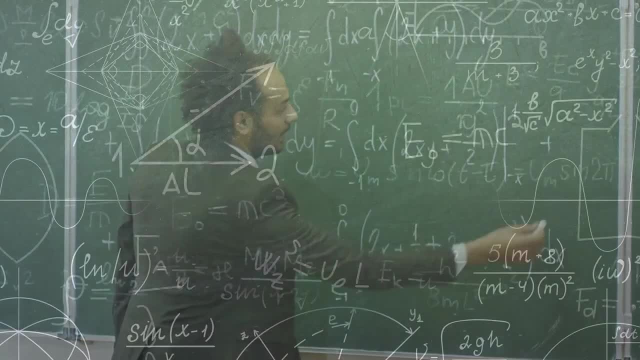 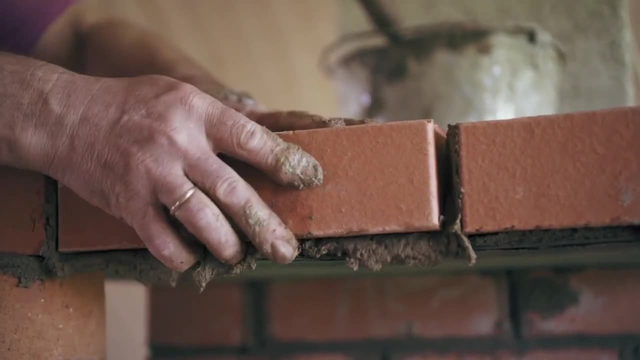 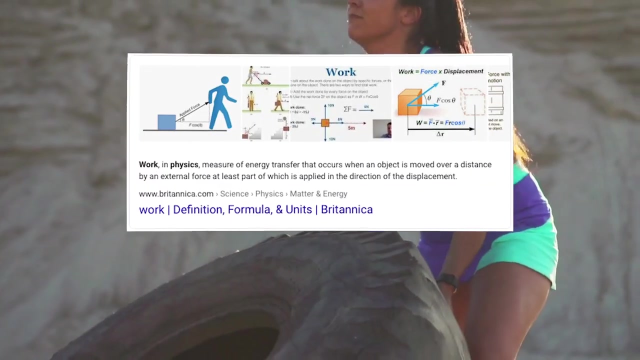 and acceleration are foundational to life as an engineer. Every other principle, like work, energy, forces, everything builds off your understanding of these concepts. So let's talk about work and energy. Work builds off the principles of force. If work is done on an 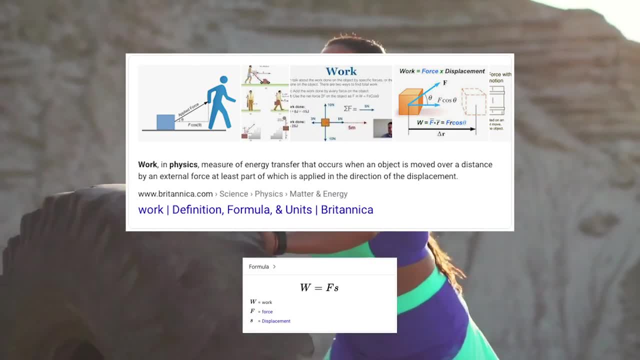 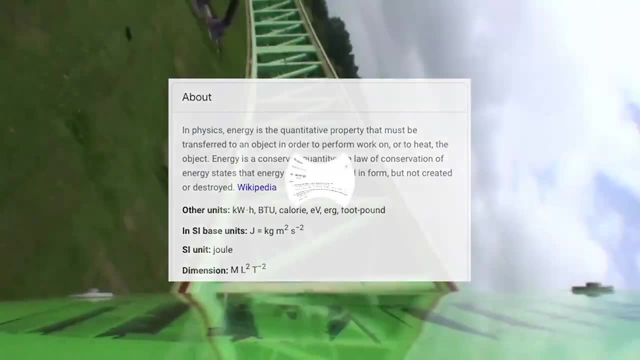 object, a force is applied to that object to move it a certain distance in a certain direction. Energy is the capacity of doing work. For example, when you're in a car, at the top of a roller coaster, you have a certain amount of energy, or potential energy, to fall down the track and gain. 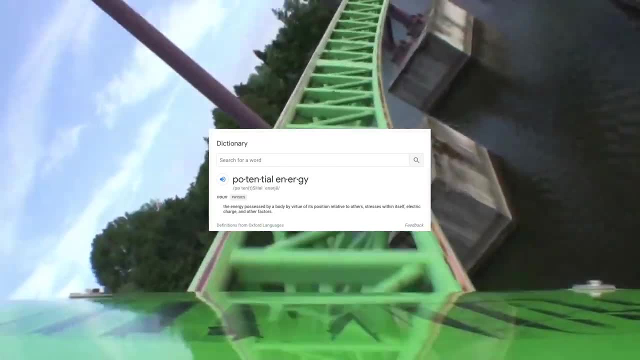 speed. If you're in a car, you have a certain amount of energy or potential energy to fall down the track and gain speed. As you begin to fall, your potential or potential energy begins to decrease as the force of gravity begins doing work on you. Think of energy as the currency. 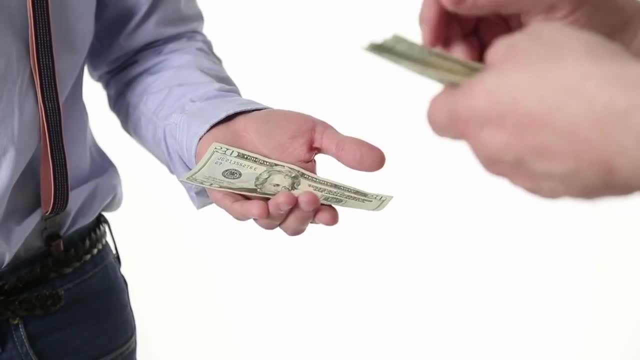 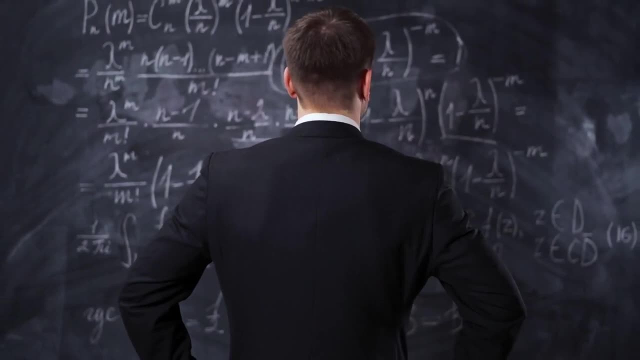 to do work. As an analogy, your manager or boss might pay you in energy and in turn, you work all day. These principles aren't hard if you understand forces and, ultimately, accelerations, but, like everything in physics, it all builds off your understanding of previous principles. 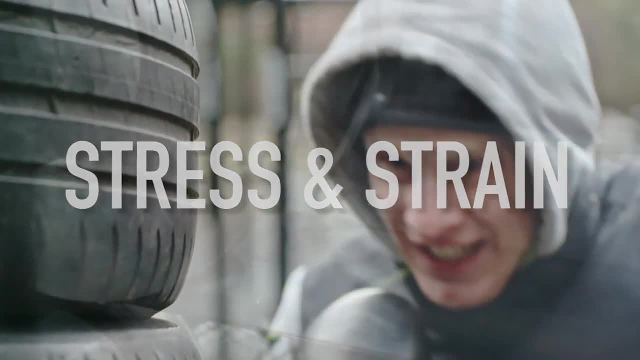 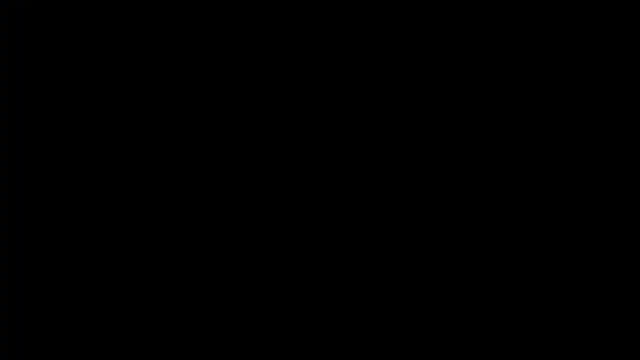 Finally, let's talk about stress and strain. Stress is the force per unit area and strain is the deviation or change in shape as a result of stress. In other words, stress is the amount of tests you have coming up when you're in school. 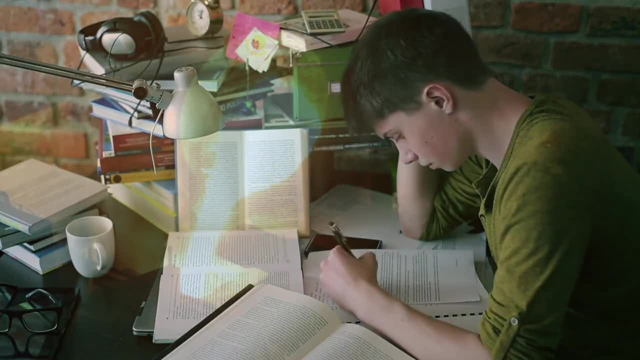 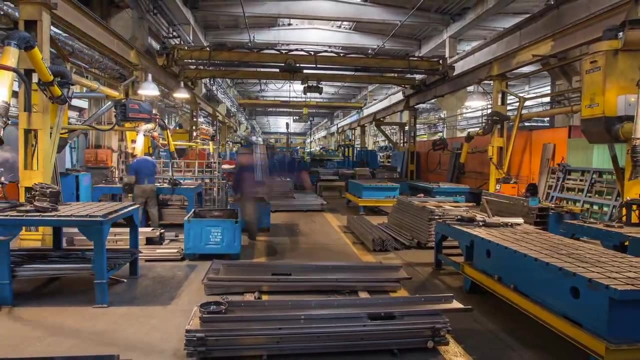 and strain is how little free time you have in your schedule. These concepts become really important in material sciences. Their values will change for different materials, often referred to as maximum stress and strain for a given material. Exceeding these maximum values often results in. 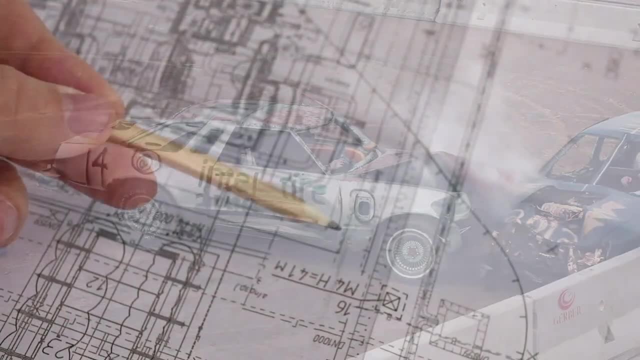 deformation or loss of energy, Stress is the force per unit area and strain is the deviation or change in shape as a result of stress or part failure. All of the concepts we just mentioned were physical in nature and they involve a lot of underlying math. too Many engineers use these. 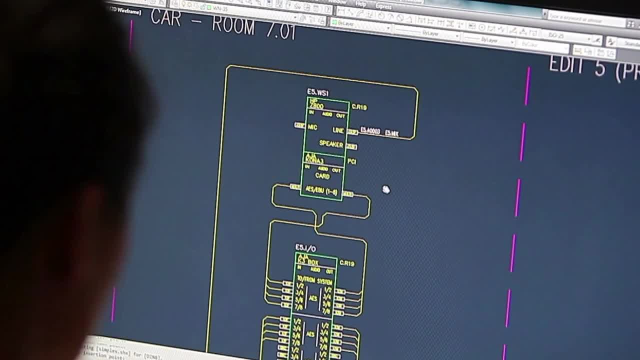 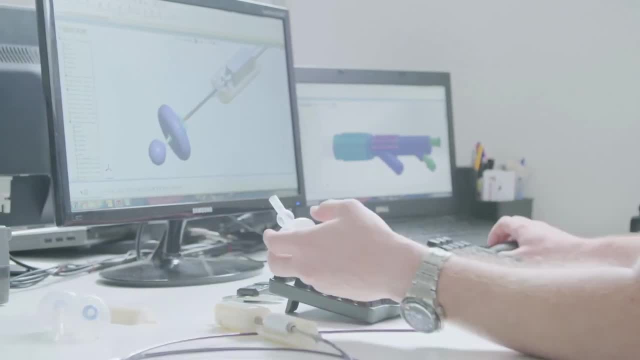 principles on a daily basis, although not always in the way you use them in physics class in high school or college. Most computer-aided design programs and other computer tools will take the complexities out of the calculations and determine all of these values automatically. for a part, that 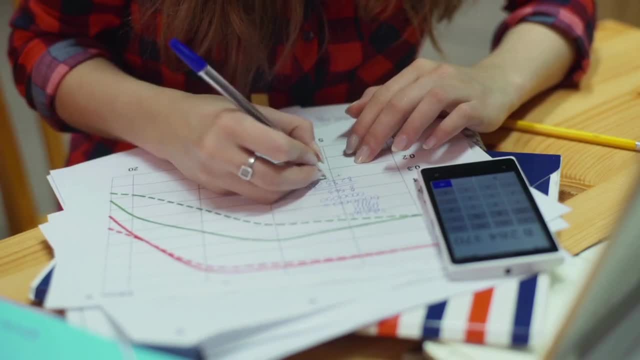 you design. That doesn't mean you don't have to understand the principles, but you do have to make the job of being an engineer just a little bit easier.